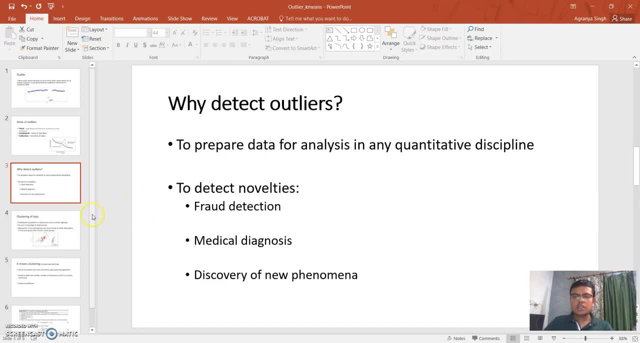 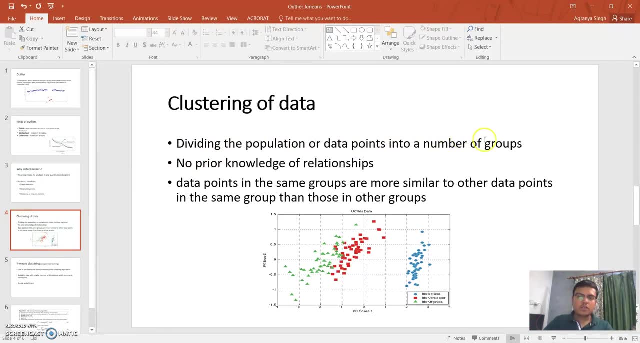 of detect outdoor detection. let's move on to clustering of data, and then we'll relate these two fields. so clustering of data. dividing the population or data points into a number of groups without any prior knowledge of relationships is clustering of data. the condition that is imposed is that the data points in a group should be more similar to the data points in that particular group. 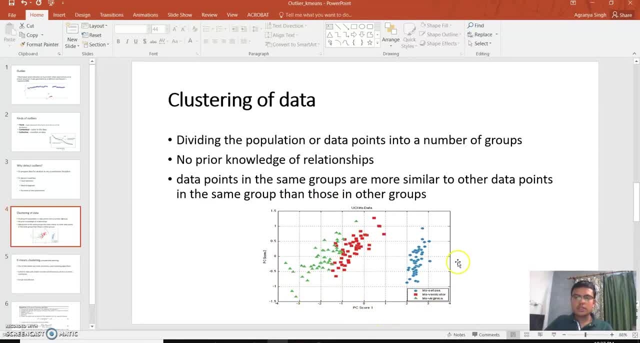 rather than those in other groups. now we can see this plot as an example of how data is clustered into three different groups based on their scores for a particular attribute. so that is how clustering is performed. now there are different algorithms present for clustering data into different groups. we'll be 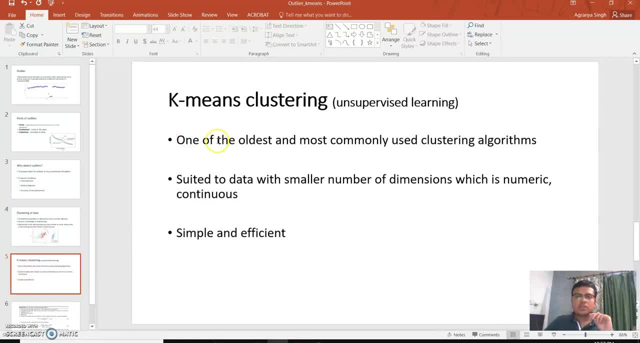 focusing on k-means clustering. so k-means clustering is an unsupervised learning algorithm which is one of the oldest and most commonly used clustering algorithms. because of its simplicity and efficiency. it is suited to data with smaller number of dimensions, which is numeric and continuous. 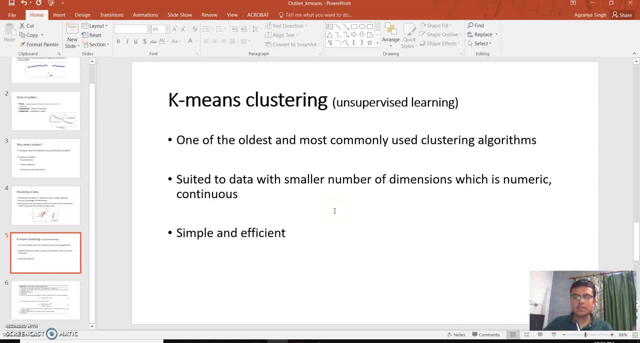 now. definitely this algorithm has its limitations because it is quite old and also efficient. so we can't quite compare its accuracy with the other algorithms. so we can't quite compare its accuracy with the more recent algorithms that are more resource intensive, but we'll see why it is still. 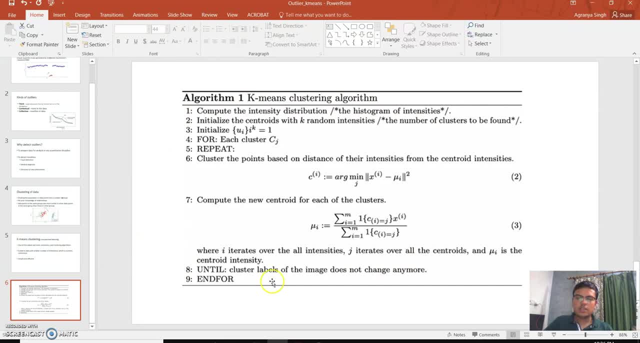 widely used and appreciated. you can have a look at this algorithm. i'll just explain in brief the steps that are required. so the first is to get the number of clusters to be found. so this is a requirement for this algorithm and also one of its drawbacks. so for that we can use the intensity. 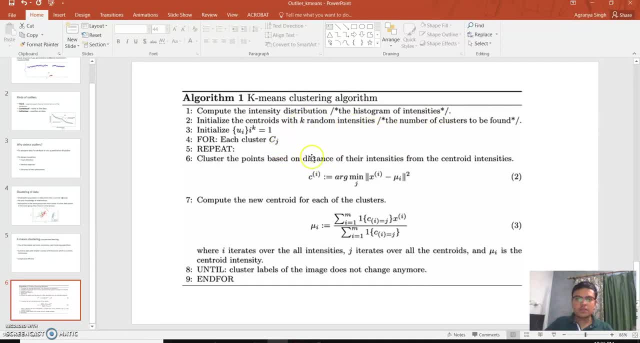 distribution and once we have found the number of clusters, we can we we initialize the cluster centers. points are clustered based on the distance of their intensities from the centroid intensity, so euclidean distance is used for this purpose. now, after each point is put into a cluster, the centroid. 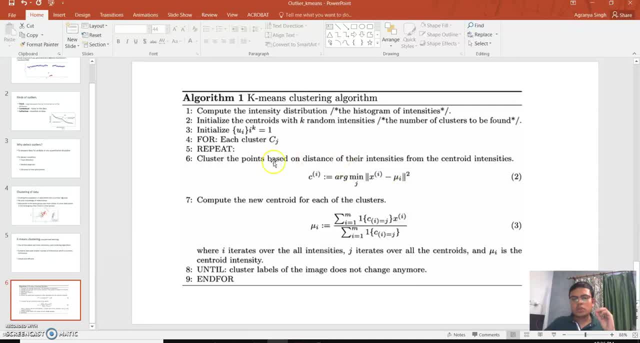 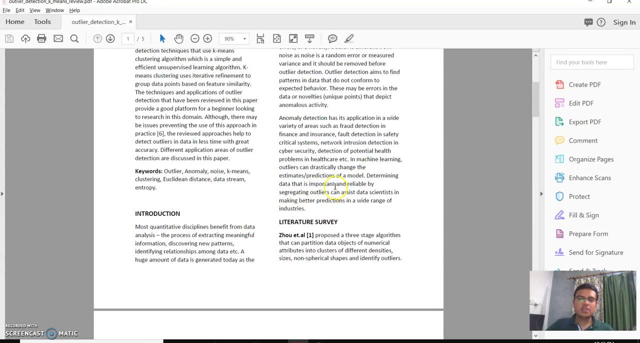 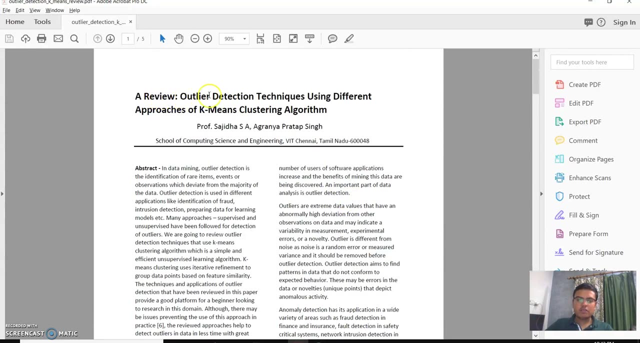 is again computed for that cluster and the process. this process is repeated until all points fall into some particular cluster. now that we have a basic idea of what is outer detection and how clustering uh works- specifically the k-means clustering algorithms- we'll move on to reviewing uh five. 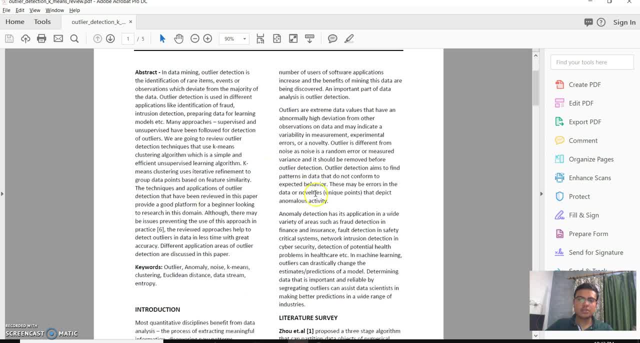 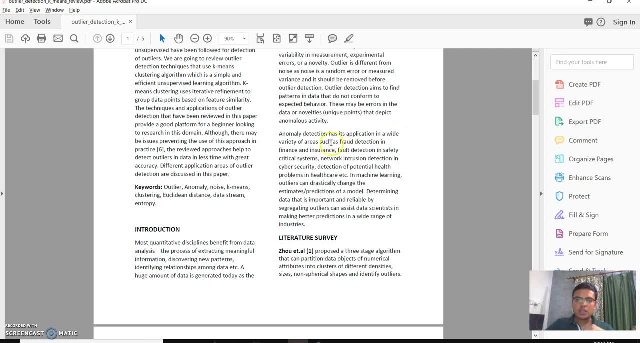 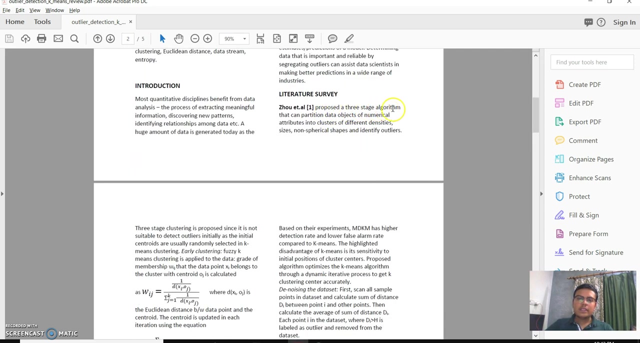 k-means clustering that are used in outlet direction. so once again, i would like to highlight the application of anomaly detection. so applications are fraud detection and finance and insurance fault detection, safety, critical systems, network intrusion detection, cyber security, so on and so forth. so, moving on to our review, the first paper that we'll review has proposed a three-stage. 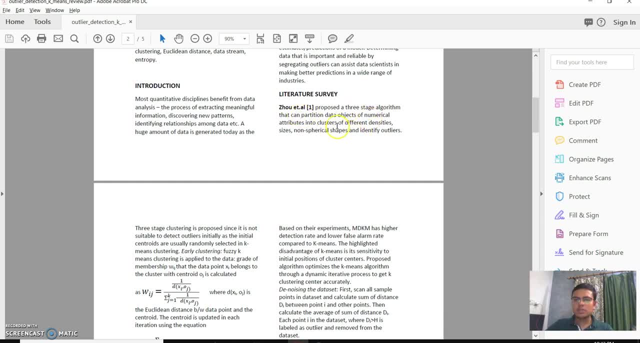 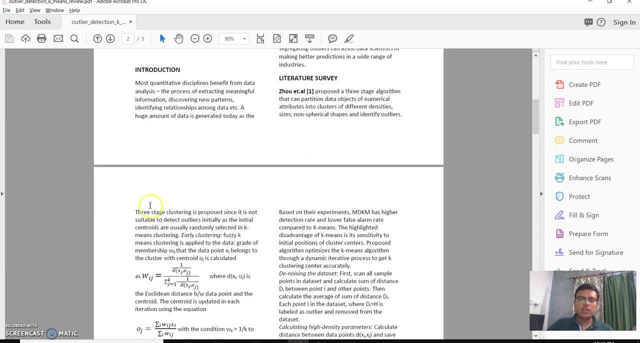 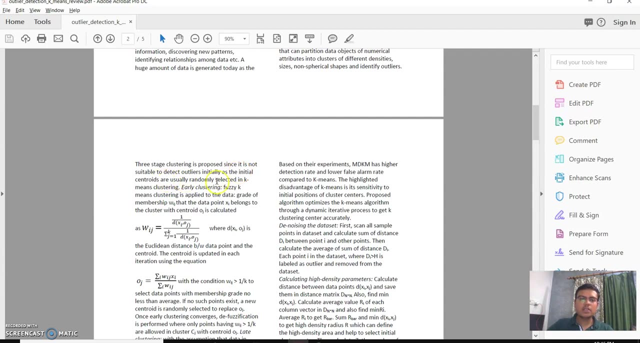 algorithm that can partition data objects of numerical attributes into clusters of different densities, sizes, even non-spherical shapes, and identify the outlet. so three-stage clustering is proposed. proposed since it is not suitable to detect outliers initially, as the initial centroids are usually randomly selected in k-means clustering. so early clustering, fuzzy. 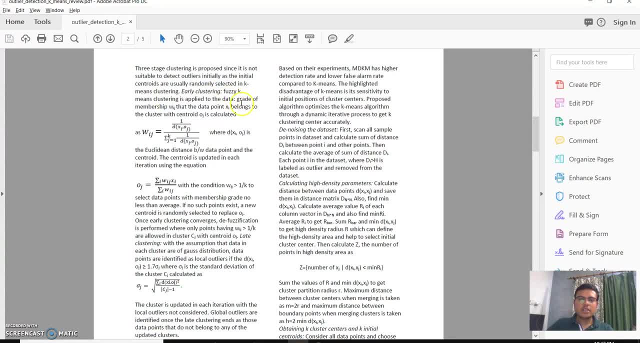 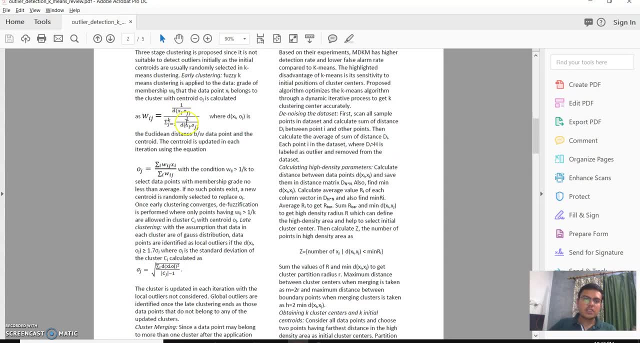 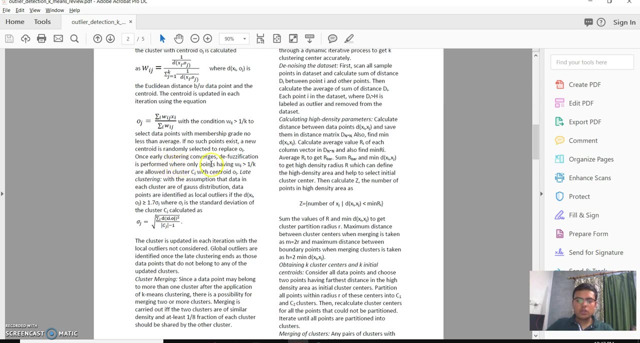 k-means. clustering is applied to the data to get the grade of membership wi according to the formula. you can go through this algorithm in detail in the research paper. once we got the grade of membership, defuzzification is performed where only points having a specific uh grade of membership are allowed in the cluster with cent, with a. 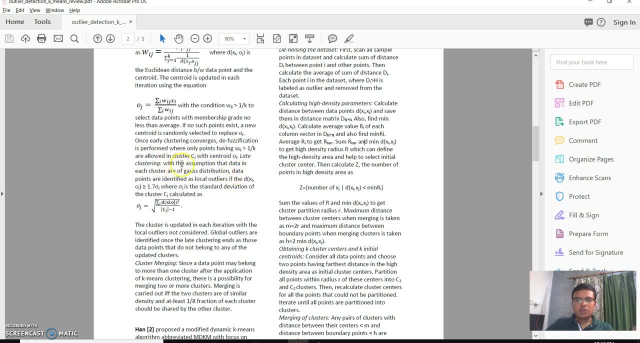 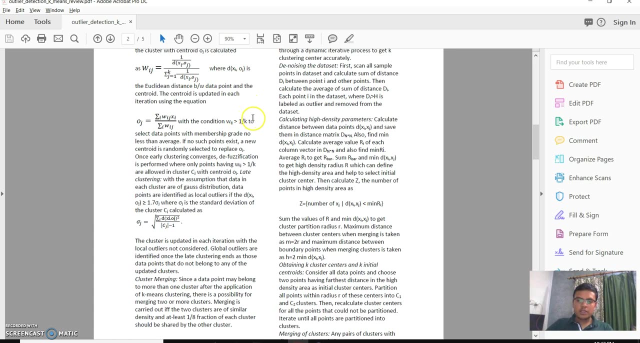 particular centroid. so in late clustering the assumption is made that data in each cluster follows gauss distribution. data points are then identified as local outlets if the xioj, that is, the distance between euclidean distance between a particular point and the centroid of the cluster to which it will be distributed, is determined in the following way: 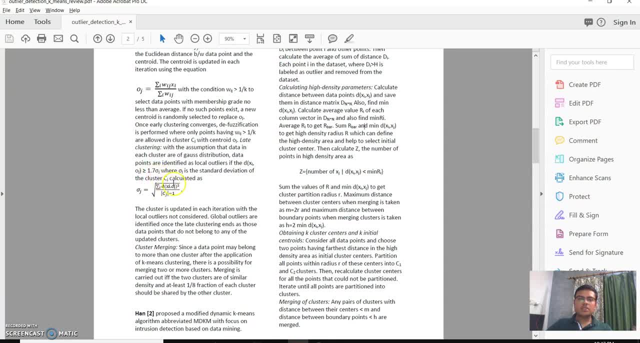 belongs is greater than 1.7, the standard deviation of the cluster that is calculated, given by this formula. So the clusters are updated in each iteration with local outlays not considered. So global outlays are identified once late clustering ends, as those data points do not. 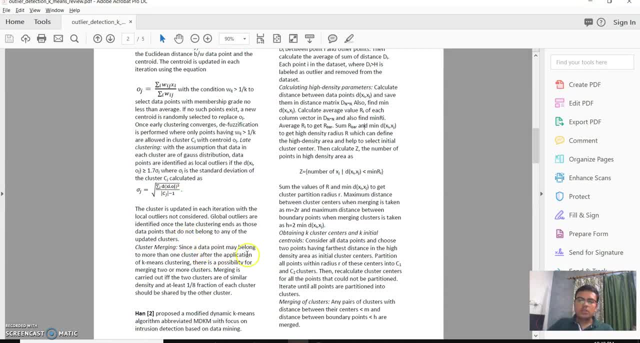 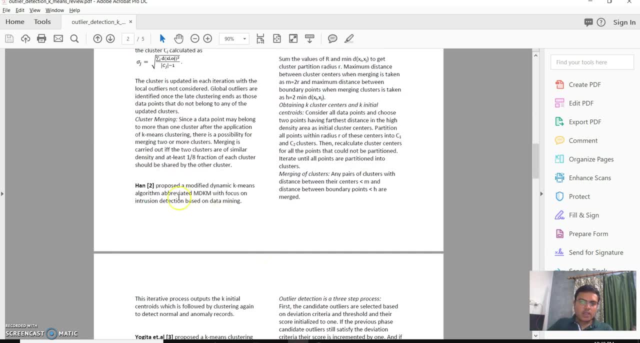 belong to any of the updated clusters. So that's how this algorithm works with regard to outlet detection. Now the next algorithm is a modified dynamic k-means algorithm, abbreviated as MDKM, with focus on intrusion detection based on data mining. So this has specific focus on intrusion detection in networks and security. 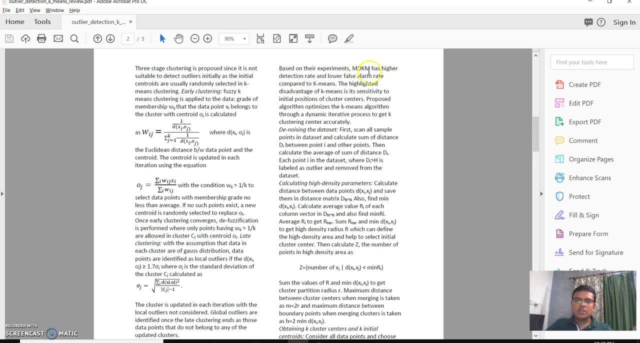 So they have tested their algorithm and, based on the results, MKDM has higher detection rate and lower false alarm rate compared to k-means. So they have tested their algorithm and, based on the results, MKDM has higher detection rate and lower false alarm rate compared to k-means. 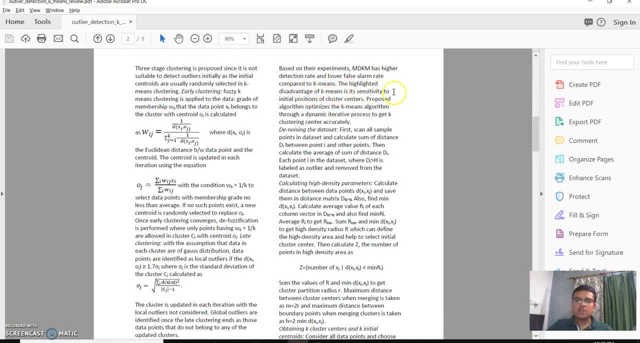 So highlighted disadvantage of k-means is sensitivity to initial position of cluster centers. that has been highlighted even in the paper that we have seen before this one. So the proposed algorithm optimizes the k-means algorithm through a dynamic iterative process to get k clustering center accurately. 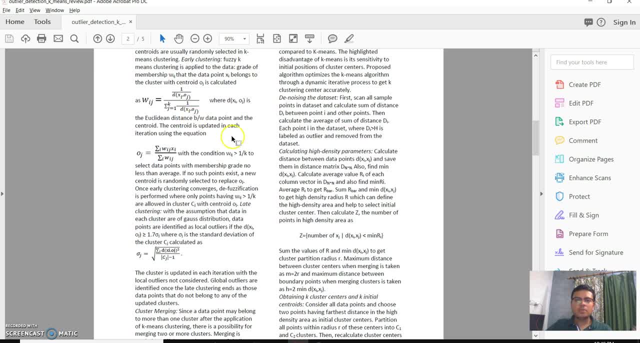 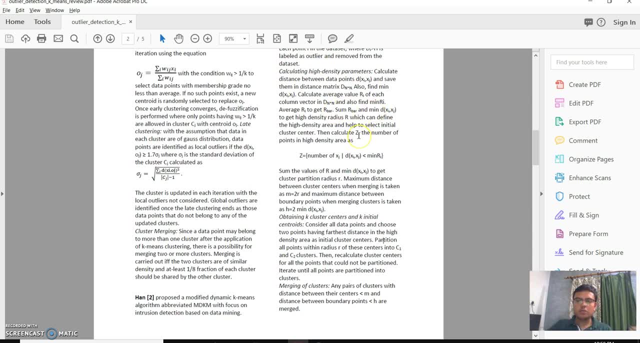 So the first step is denoising the dataset that is common to most of the algorithms that we are going to look at. So the next step involves calculating high density parameters, that is, the high density area and the number of points present. So once we have got the high density parameters, we proceed with clustering. 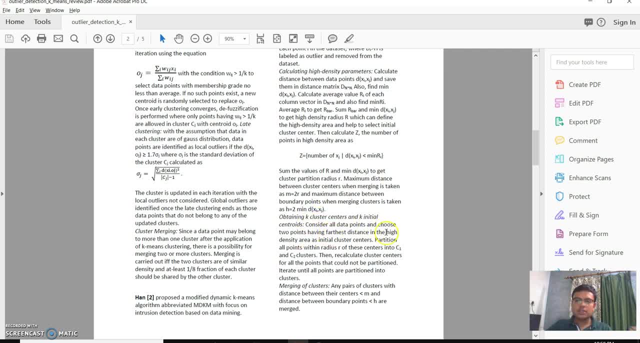 So we consider all data points and choose two points having farthest distance in the high density area as the initial cluster centers. Then we partition all points within radius R of these centers into C1 and C2 clusters. So the two farthest points form two different clusters, C1 and C2.. 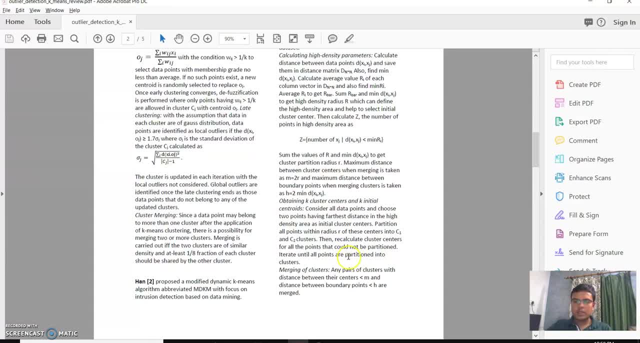 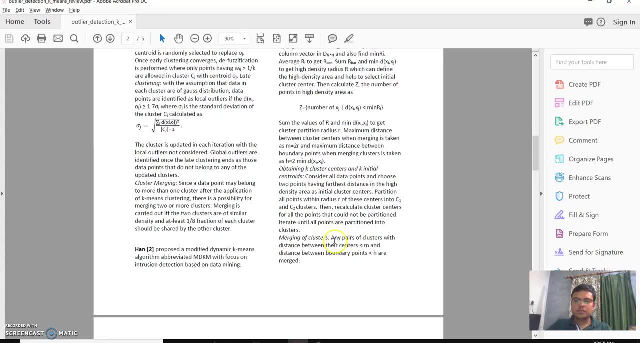 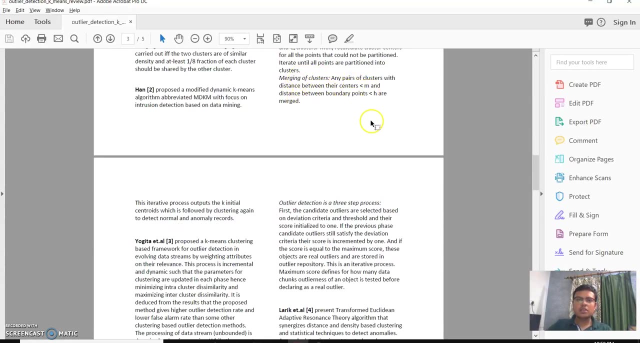 Then we can recalculate the cluster centers for all points that could not be partitioned. This whole process is an iterative process that repeats until clusters are formed and then merging of clusters is performed based on this condition. After this we can detect the outliers based on the clusters, and the points that are not. 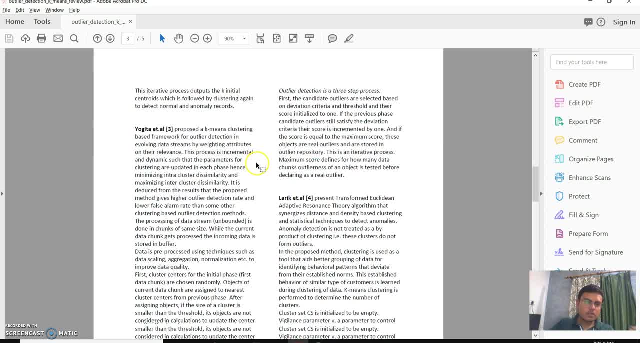 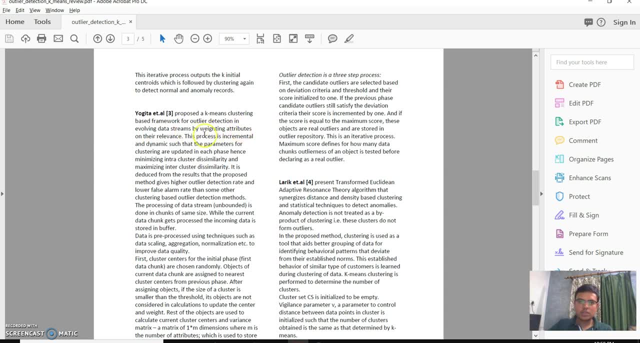 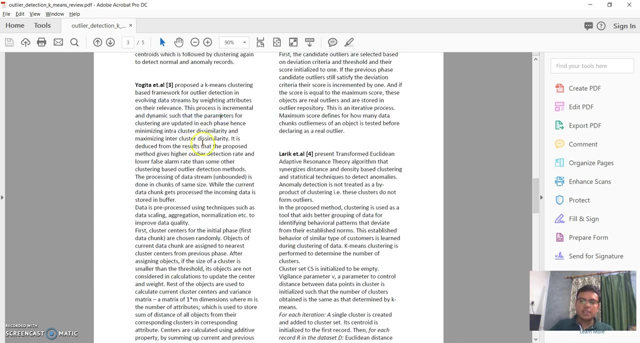 present in any cluster can be termed as outliers. So the next paper that we will look at proposes a k-means clustering based framework for outlier detection in evolving data streams by weighing attributes. So this is specifically for evolving data streams. Now this is an incremental and dynamic process, such that the parameters for clustering are 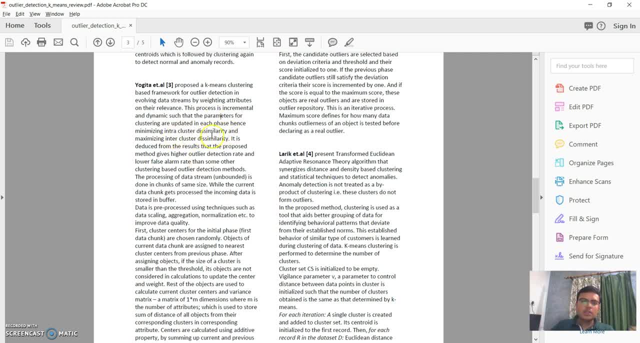 updated in each phase, Hence minimizing intra-cluster dissimilarity and maximizing inter-cluster dissimilarity, So hence increasing the efficiency of k-means clustering. So the processing of data stream, which is unbounded, is done in chunks of same size. While the current data chunk gets processed, the incoming data is stored in a buffer. 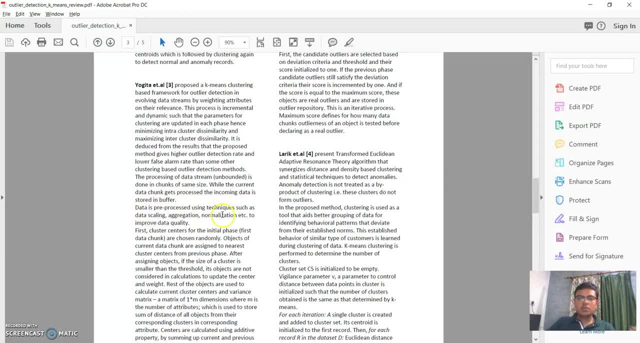 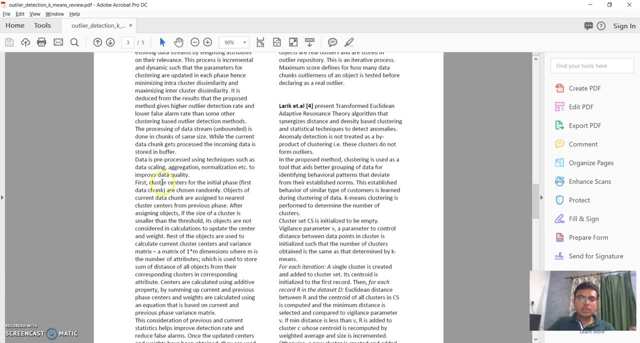 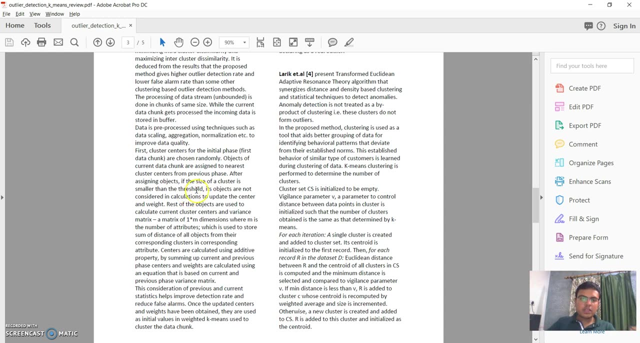 Again, data is preprocessed using techniques such as data scaling, aggregation, normalization, etc. To improve the quality of data. Now the steps of this algorithm proceed as follows. The first step in the initial phase is to choose the cluster centers randomly. Again, for the further upcoming phases, the cluster centers are calculated using summation. 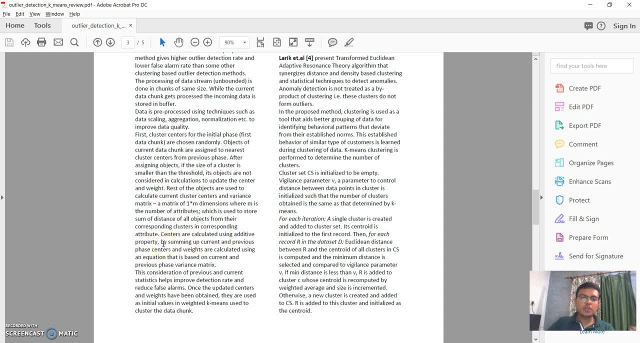 that is, centers are calculated using additive property by summing up current and previous phase. centers and weights are calculated using an equation that is based on current and previous phase variance matrix. Now, what is a variance matrix is defined here. a matrix of 1 is to m dimensions, where m is. 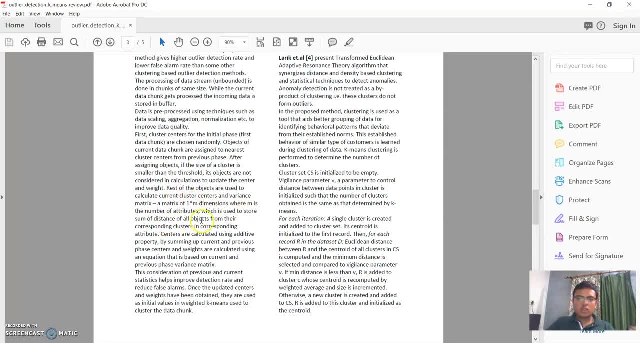 number of attributes, which is used to store sum of distance of all objects from their corresponding clusters and corresponding attribute. Now, since this algorithm updates these parameters, that is, the cluster centers and the weights, at each new phase. So this is an dynamic algorithm and the dynamic nature of this algorithm helps improve detection. 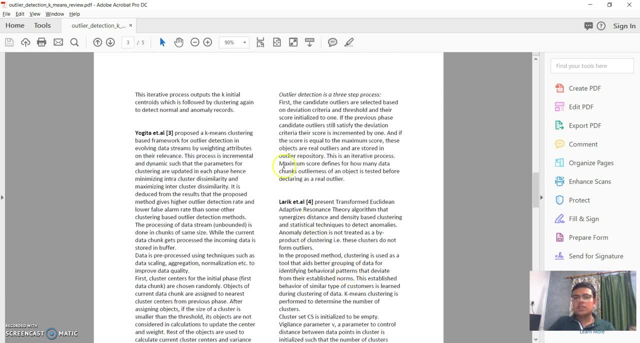 rate and reduce false alarms. So outlet detection again is a 3 step process. candidate outliers are selected based on deviation criteria and threshold and their score is initialized to 1. So at each like once. if the previous phase candidate outliers still satisfy the deviation criteria in the next phase, then their score is incremented and once the maximum score. 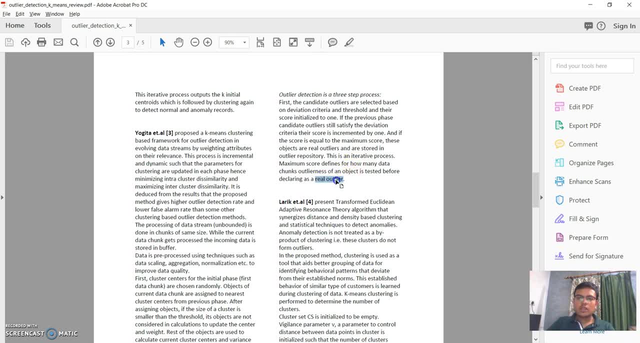 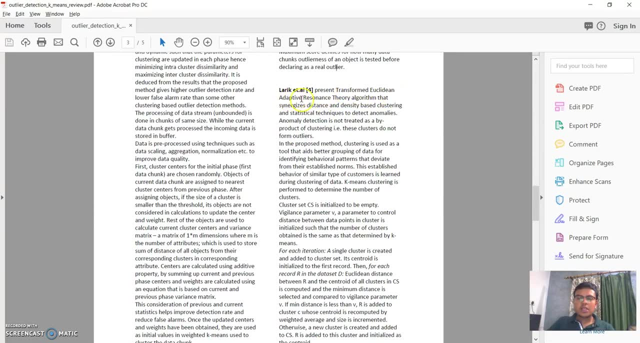 is reached, then they are declared as a real outlier. So that is how this algorithm proceeds. Now the next one, Previous phase. Previous phase Present a mushroom nuclear and that adaptive resonance theory algorithm that synergizes that system said they'd asleep is spent, and statistical techniques toечатın from this. 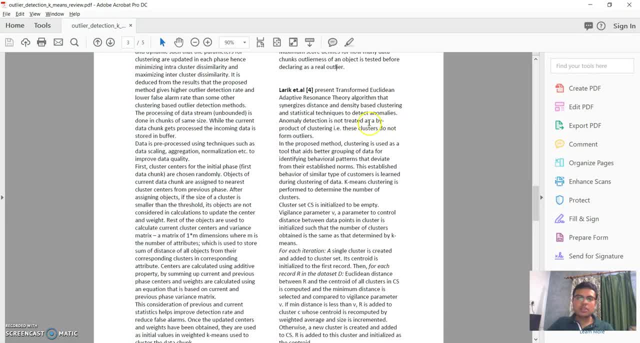 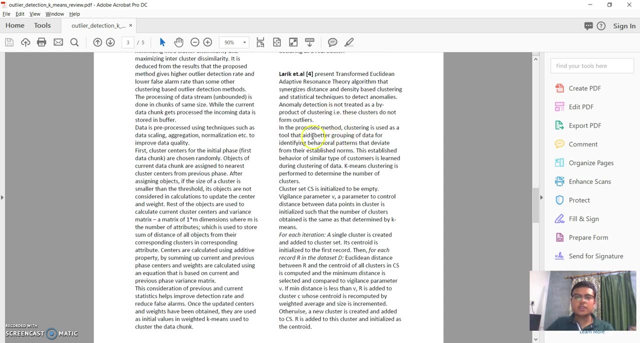 is this does not simply rely on k means it it more specifically, the horizon and adaptors during, And k means this basically used to get the initial idea of the clusters in This algorithm also does an estimate, which is this I would use as an example. 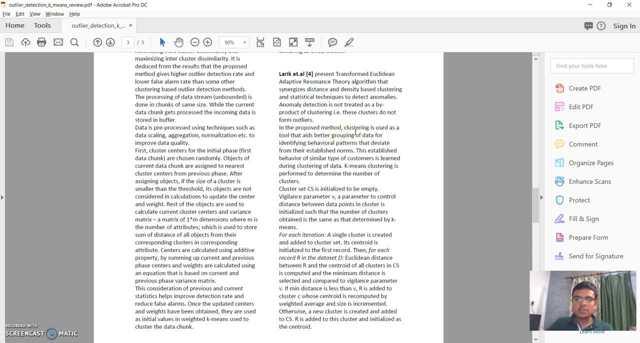 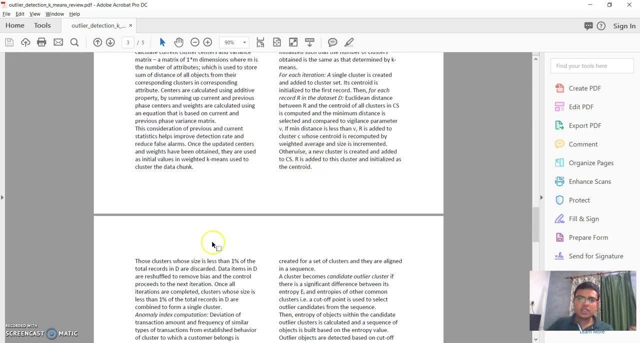 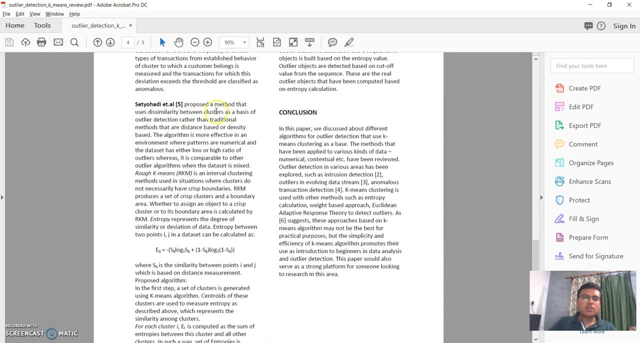 algorithm is applied to anomalous transaction detection and has produced decent results in that domain. so we'll not get into the details of this algorithm, because you can have the paper. you can read the paper for that now. the next method uses entropy based calculation to detect outliers, rather. 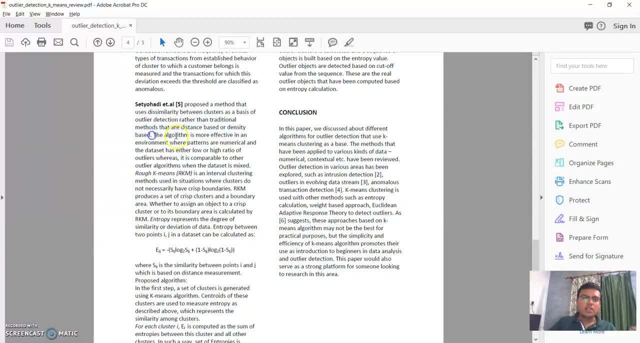 than traditional methods which are distance based or density based. so the algorithm based on the results is more effective in an environment where patterns and numerical and data side is lower. high ratio of outliers, whereas there's also comparable to other outlet detection algorithms from the data set is mixed. so rough k-means algorithm which is interval clustering method used.